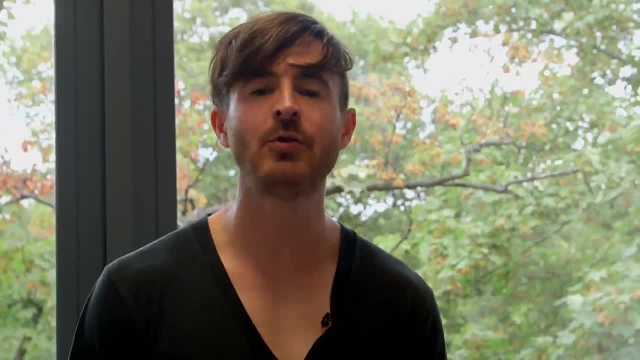 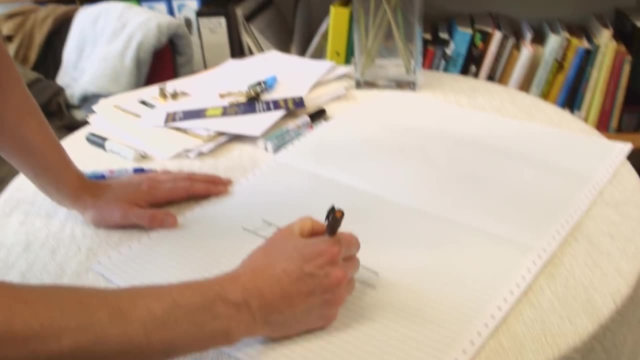 You have a way of writing down information in a coded form. His way was to think of a tape which is as long as it needs to be. It's divided up into squares, And on each of these squares there's either a 1 or a 0, or we can have some spaces. 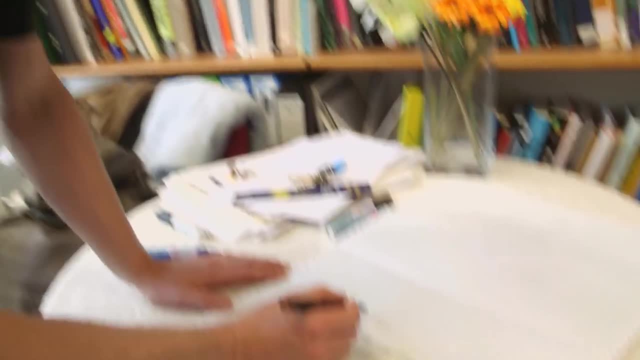 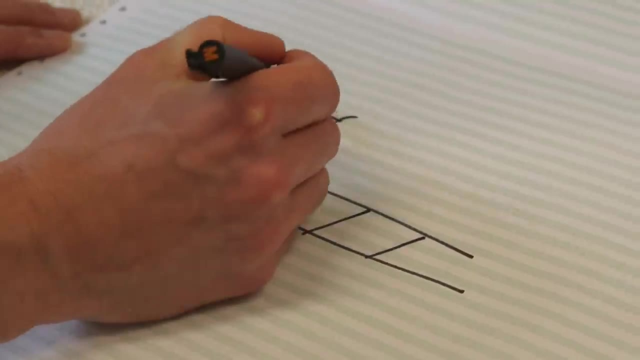 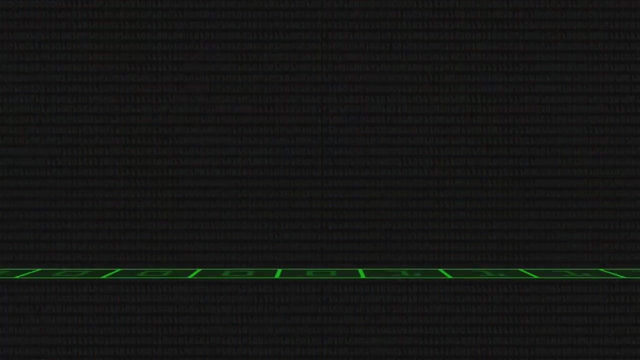 Now what our machine does is it looks at the tape One square at a time, So you could imagine it as a little box running above the tape, maybe on little wheels, looking one square at a time, And that information codes up a question or a problem that we want solved. 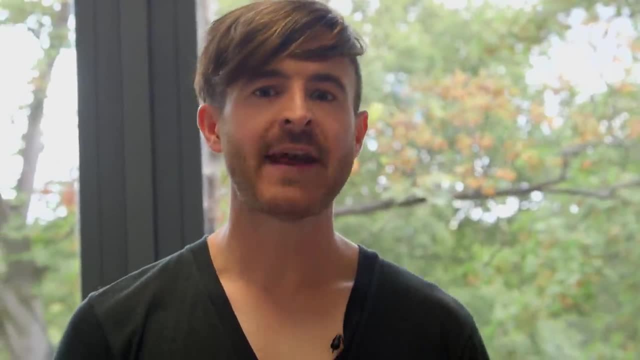 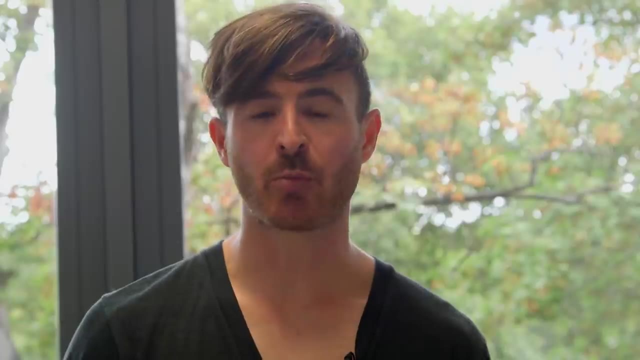 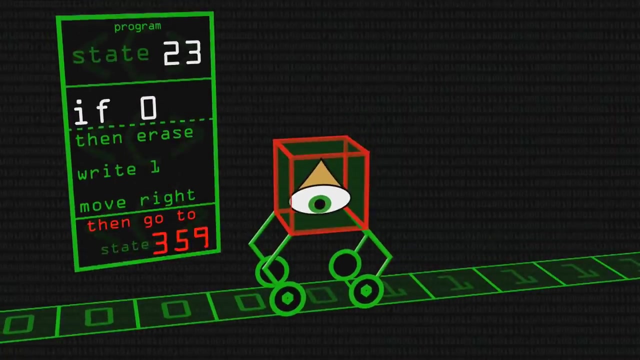 What the Turing machine does is really simple. At any moment in time, it's in a particular state and it's looking at one square on the tape And it has a logbook, A program book, And that tells it. if, for instance, you're in state number 23, and you're looking at a 0,. 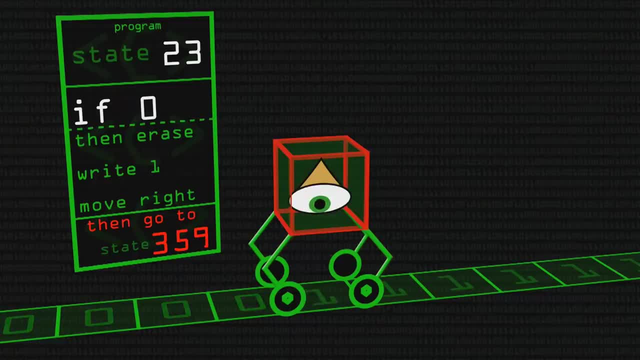 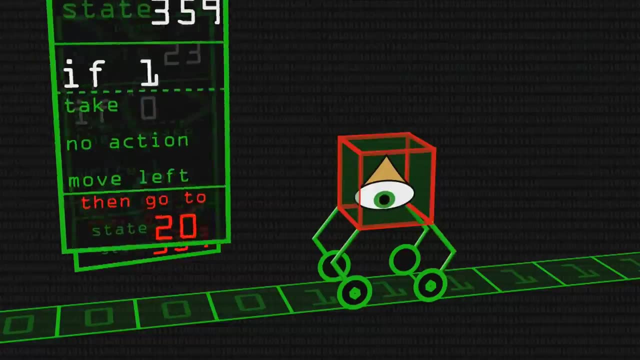 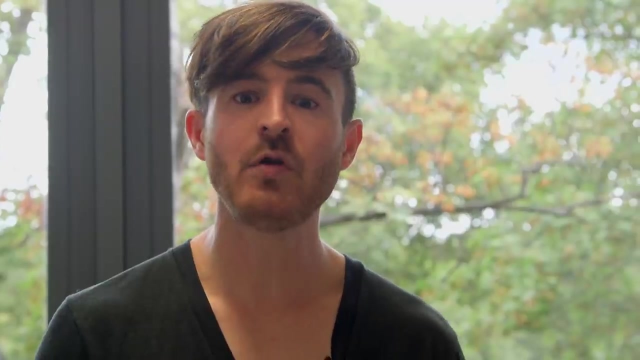 then rub out the 0, change it to a 1, move one square to the right and move into state number 359, for instance. Or if you're in state number 359 and you're looking at a 1, leave that 1 as it is, move one square to the left and move into state number 20.. 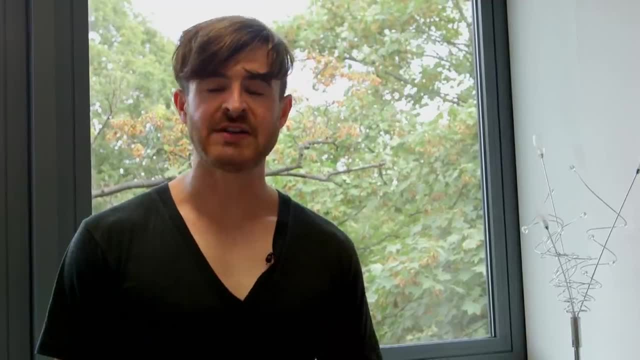 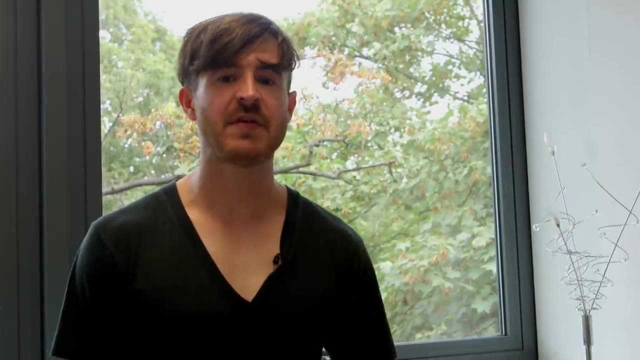 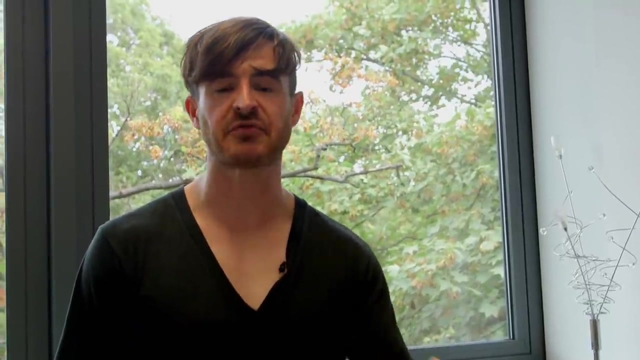 Really simple instructions. What the machine does is it starts off with a certain pattern of 1s and 0s. It follows these rules, one square at a time, transforming that string of 1s and 0s into a different string of 1s and 0s. 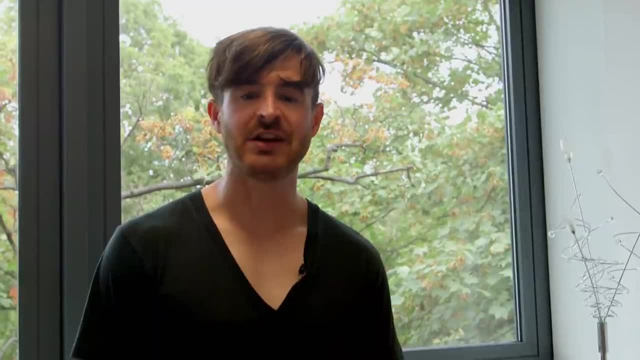 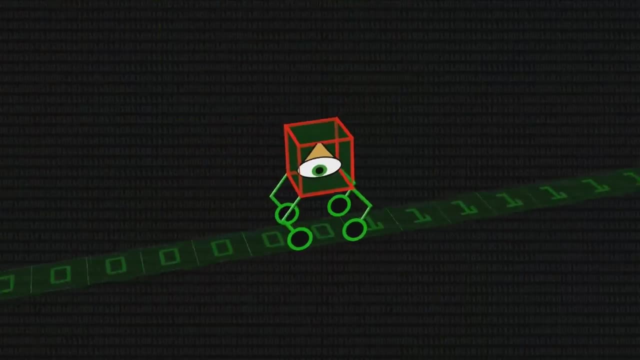 And eventually, hopefully, the machine moves into a halting state. It's finished, It's done, And what's left on the tape is the answer to our problem, coded up as 1s and 0s. That is such a simple process. 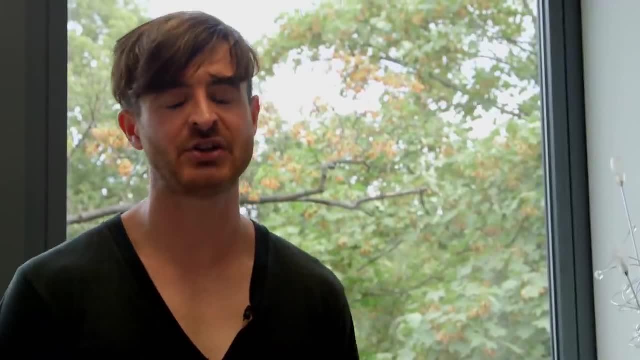 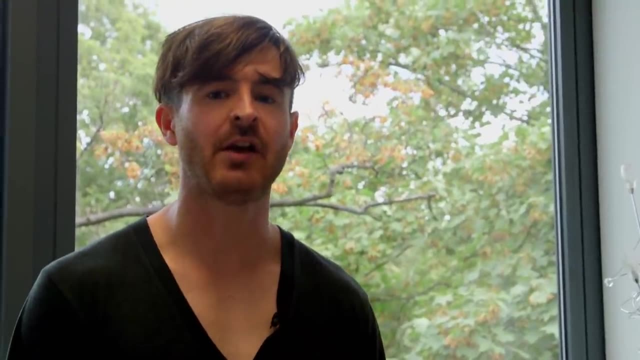 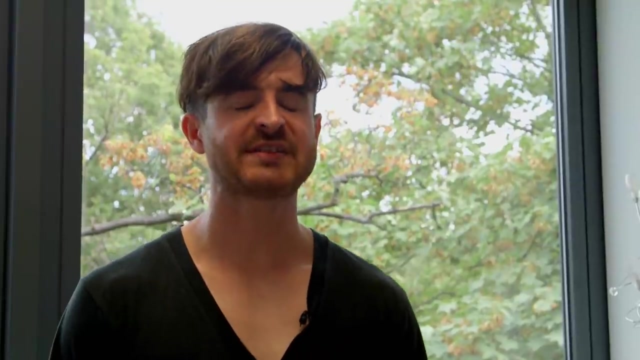 but it turns out it's the essence of computation. Whatever any computer can do, it could in theory be done by that system, looking at 1s and 0s on a tape. So that's why we say that Turing in coming up with this idea of Turing machines.